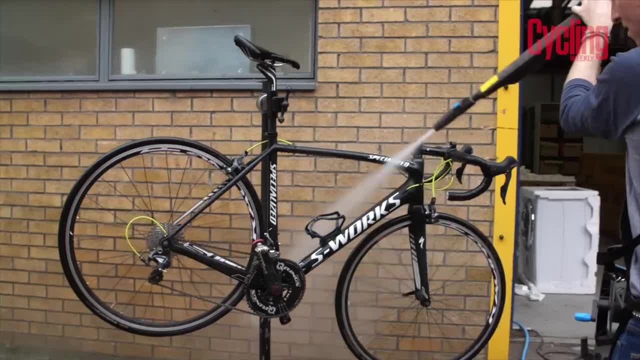 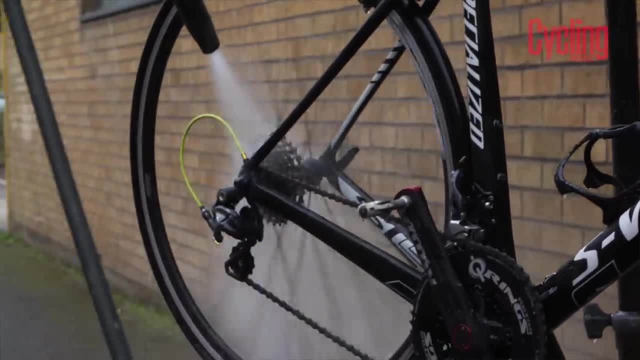 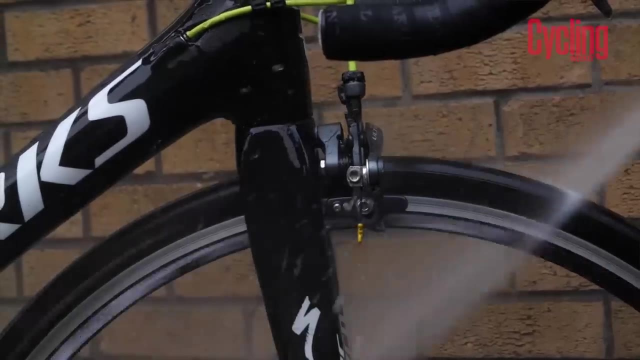 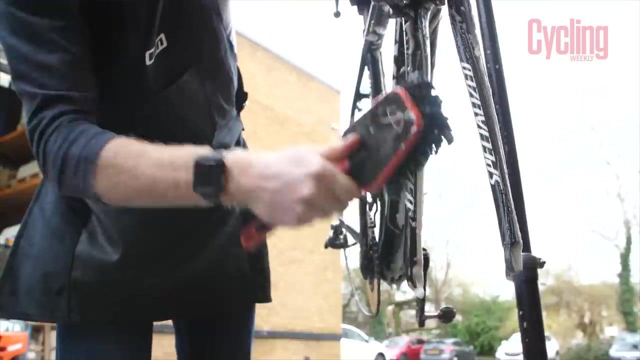 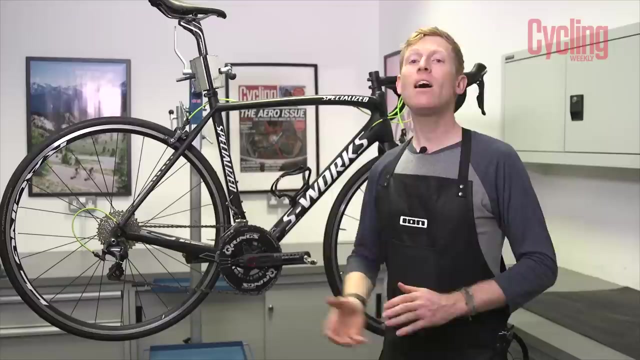 So where do you start? Well, a clean bike is a happy bike, as the saying goes. So the first thing you need to do is to thoroughly clean and degrease your bike. This will make the job of inspecting all of your components for any wear so much easier. Once it's clean, then it's time to 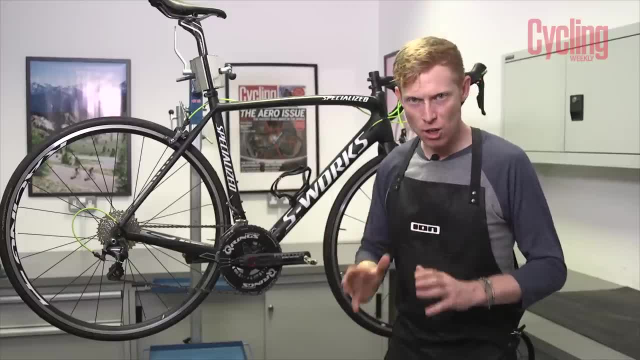 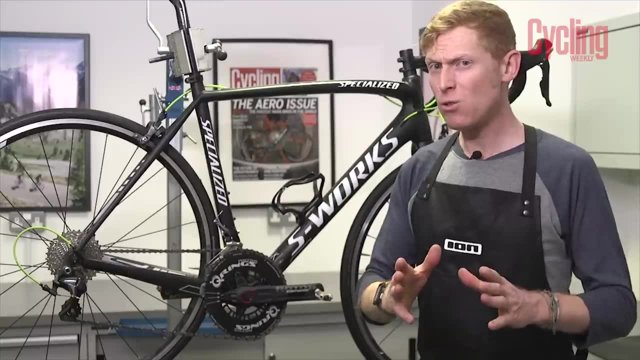 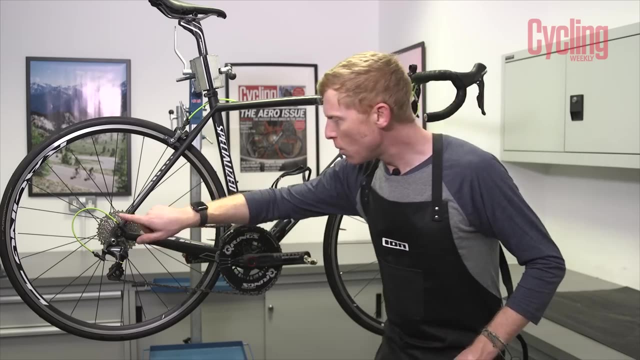 do the inspection to check that everything is good to go. Now our top tip here is to think of the capital letter M. Sounds strange, but it will help you to remember to check every single part of the bike. So the way we do it: if you draw a letter M, start from this part. here we go. look a letter M, I know it's a. 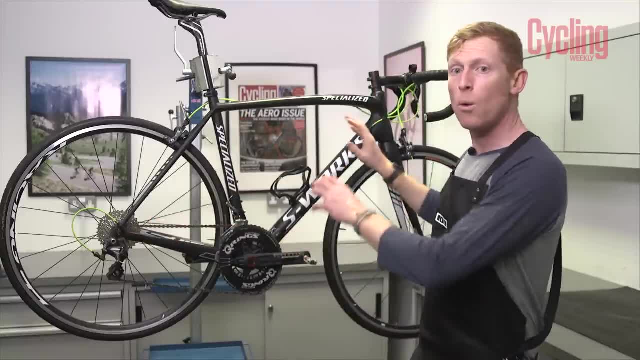 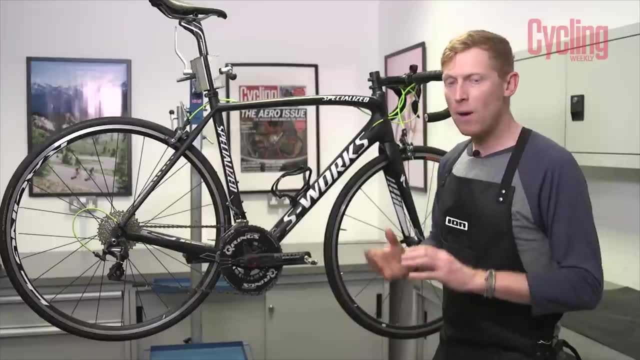 little bit weird, but this: if you follow that pattern, we'll make sure that you can check every single part. The first thing we're going to do is we're going to look at the front wheel. Now, it's really simple. We're going to check the tire first of all. So what we're 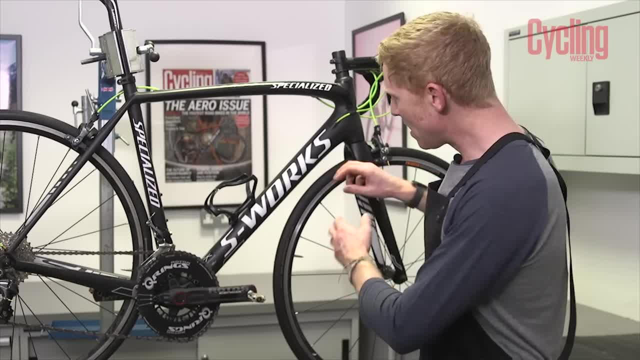 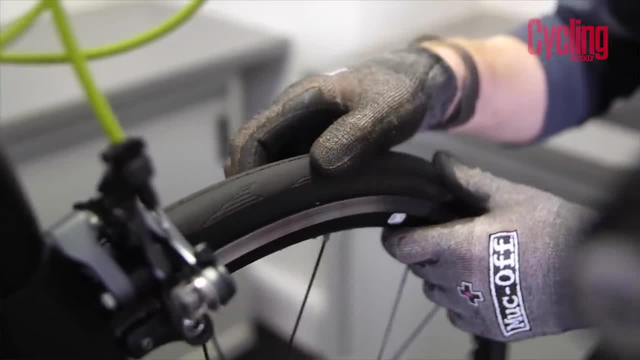 looking for here is we're looking for any damage of the tire. any little nicks that flints can cause. that could potentially cause a puncture in the future and also for any wear. So if your tire is worn, it could be a good time to change the tire as well If you're running tubeless. one of 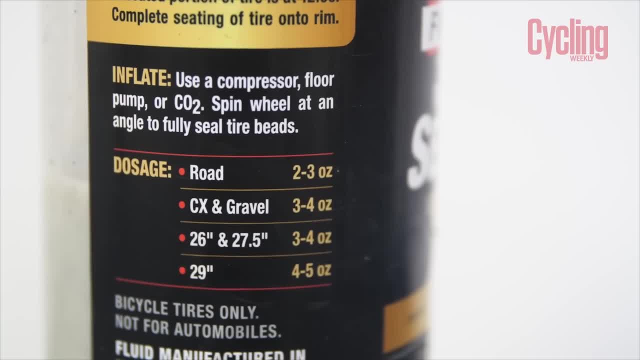 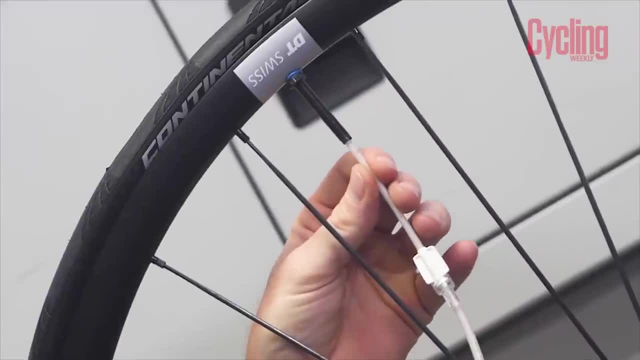 the things you need to think about as well is your sealant. So if you've not checked your sealant quantities in a while, then it's important that you do so, because sealant does dry over time, So you will need to clean it out and 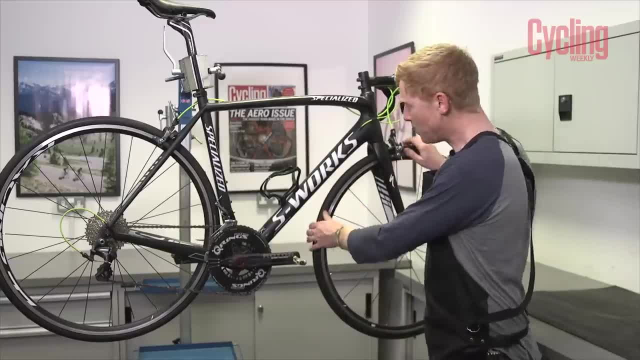 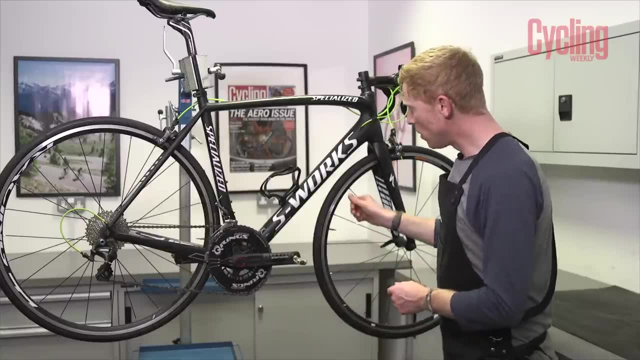 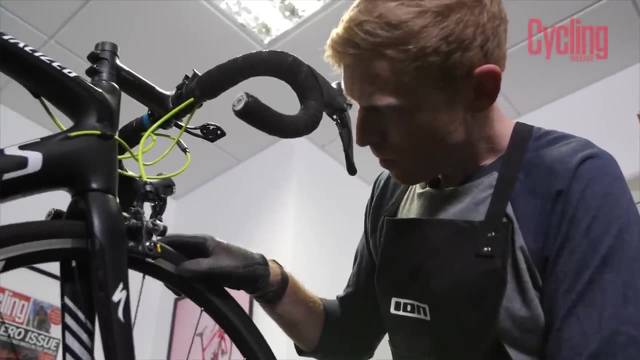 put some new sealant in. So once you've checked your tire, then you want to look at your rim. Now, this one here is a rim brake, so your rims will wear And we want to check that the rims themselves have even amounts of wear and they are nice and flat sided So there's not a concave. 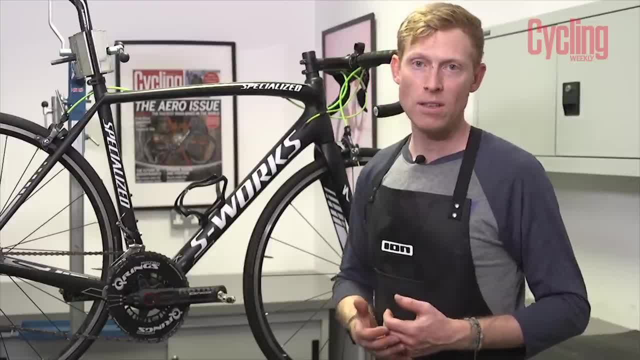 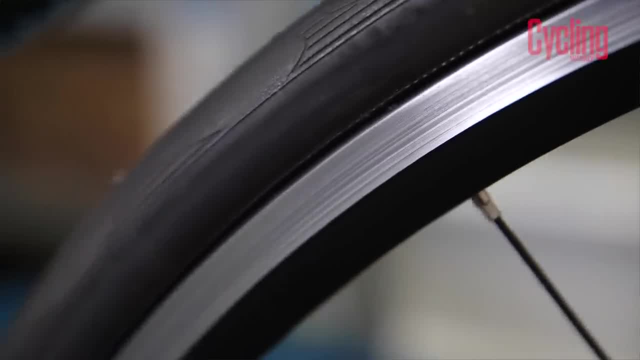 profile to that rim. That can happen when you use your brakes quite a lot If it's really concave. so if you can feel that going in, then that could be some serious damage to the rim. So you might need to check that out as well. So if you're running tubeless, one of the things you need to 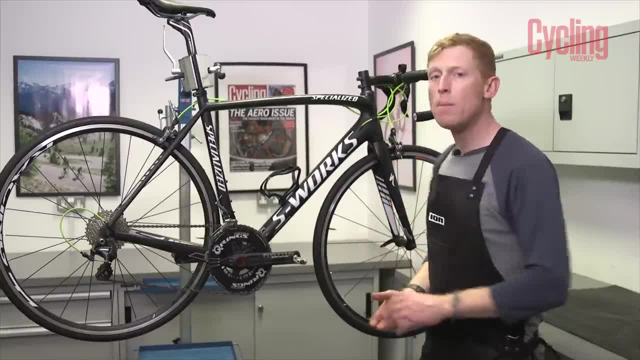 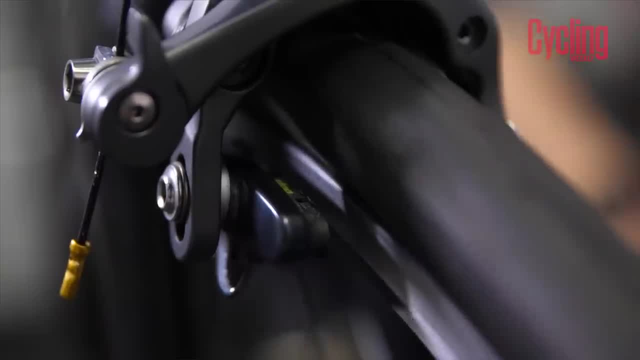 replace that. Going on from there, once you've gone past the rim, then obviously we're thinking about the wheel as a whole. So give it a spin. When you give the wheel a spin, you are going to be checking to see how true the wheel is. If your wheel is buckled, if there is a wobble in that. 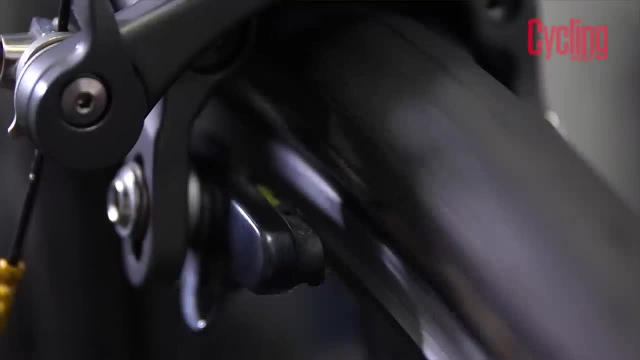 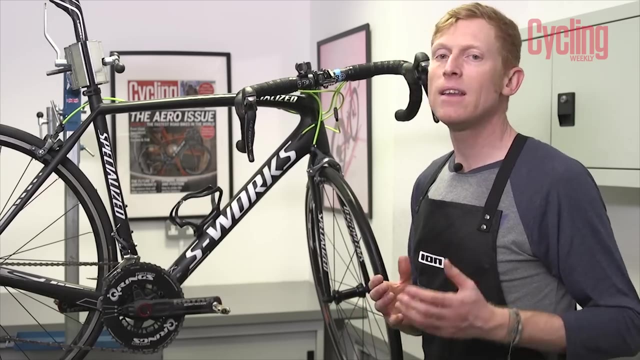 wheel. it's going to need to be sorted, Especially with rim brakes. you need to make sure that your rims are very, very true. You can do this at home, Obviously, if you are competent and happy to do so. you can check your spoke tension. You can check your spoke tension. you can check your wheel. 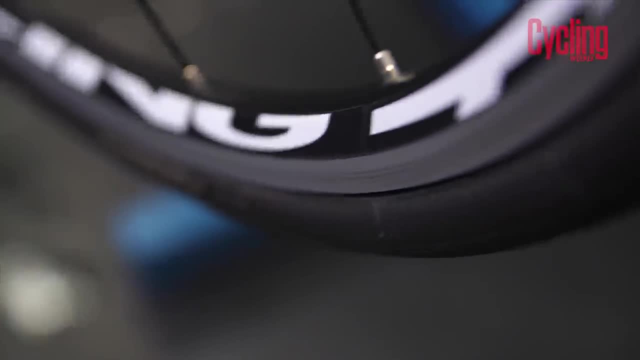 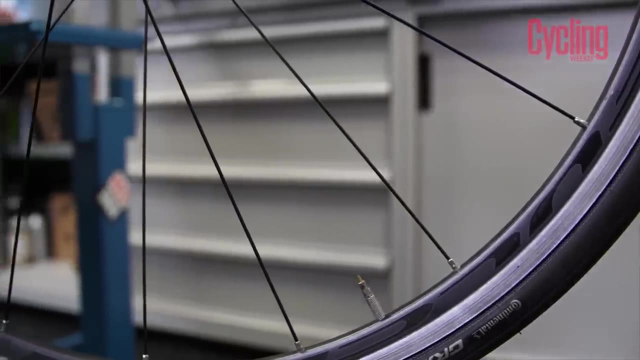 and retrue the wheels. And then, talking about spokes as well, give them a visual inspection, Have a look for any damage to the spokes, Have a look for any corrosion around the nipples themselves as well. If there is anything, then again you might need to replace parts or at 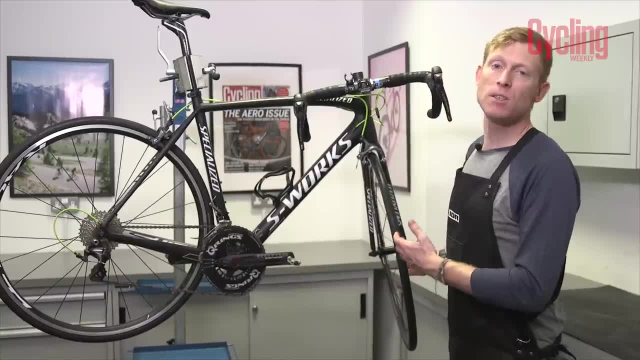 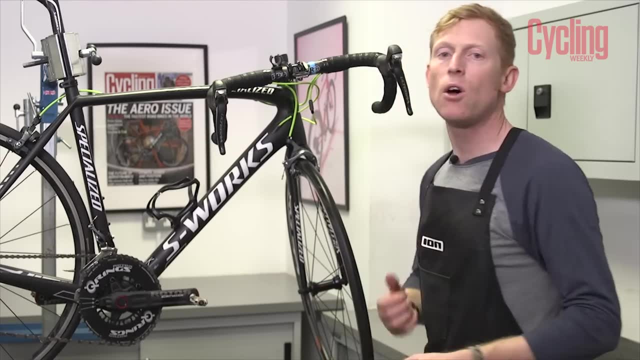 least give them a good clean. Then, finally, the most important part of the wheel, the hub itself. So we're talking about the bearings here. It spins on two bearings, on the front wheel, So you want to make sure that first of all they spin nice and freely. So there's. 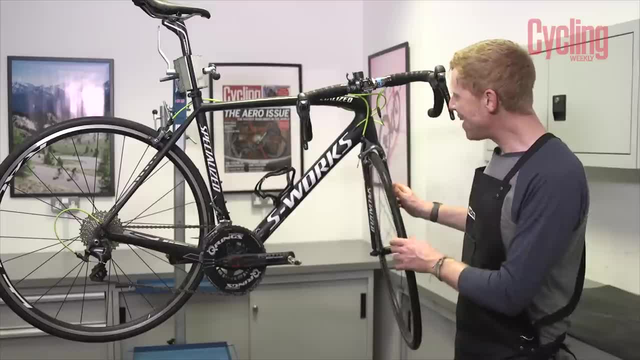 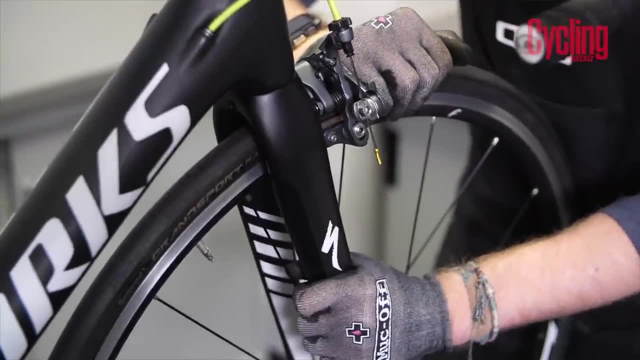 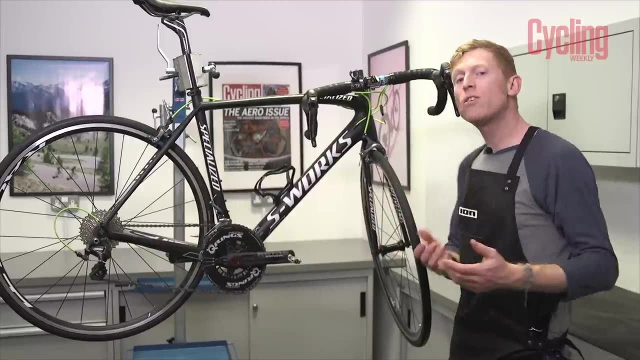 no horrible rubbing or grunching noises. And then secondly, that they're nice and tight. So if you hold onto your fork and you move that rim side to side, you're feeling for any play in the hub at either side here when it's clamped into the wheel itself. Don't try and do it out of. 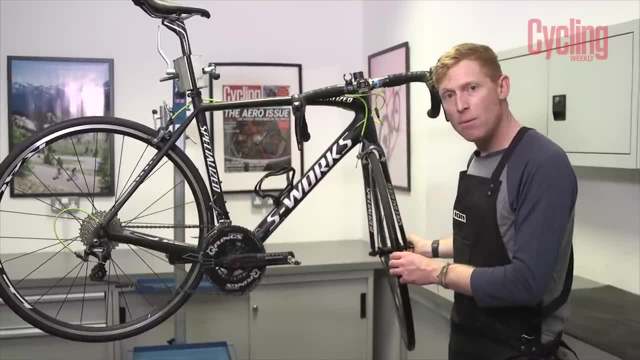 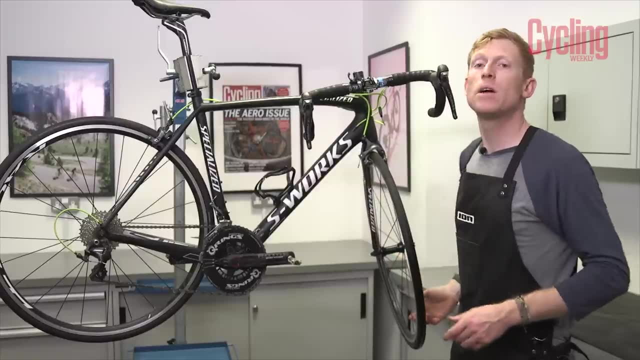 the bike because you won't feel it, Whereas if it's clamped in using the quick release, then you'll be able to notice if there's any knocking or any play in there. If, like these Fulcrum wheels, that is the case, then they are sealed bearings. You need to replace those bearings. You can't. 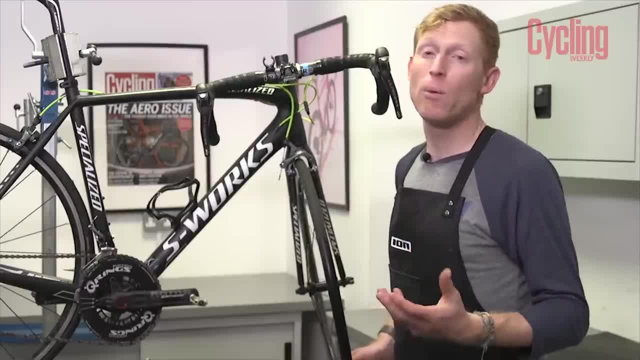 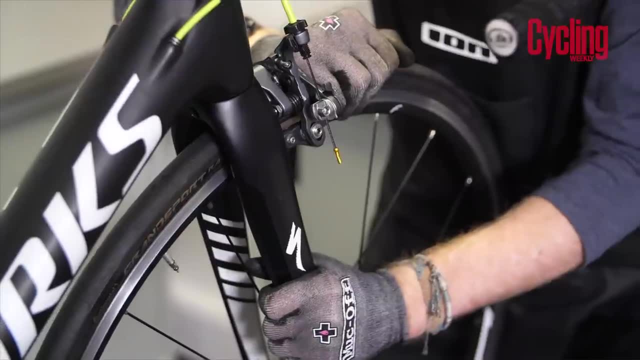 really re-tension them too much. If it's a cup and cone bearing wheel, like a Shimano wheel, then you can replace the bearings easily and you can tighten them as well. So once you've checked that the bearings are okay, you can re-grease and re-tighten As you work your way. 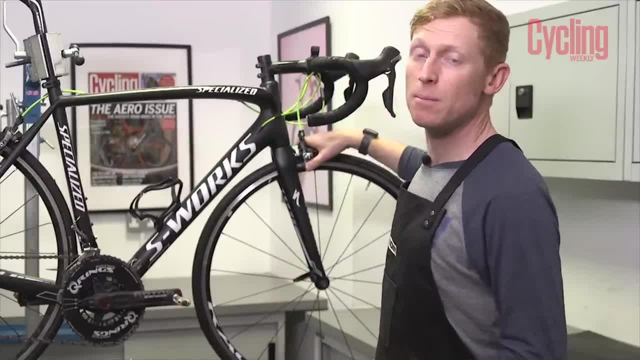 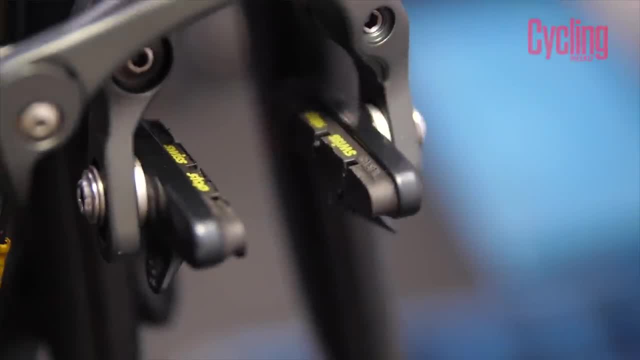 up past the wheel. then obviously we get into the brake system. Now I've got rim brakes on this. You might have disc brakes, but the same thing applies. You want to be checking your pads and you want to be checking the alignment as well, to make sure that they are working properly. 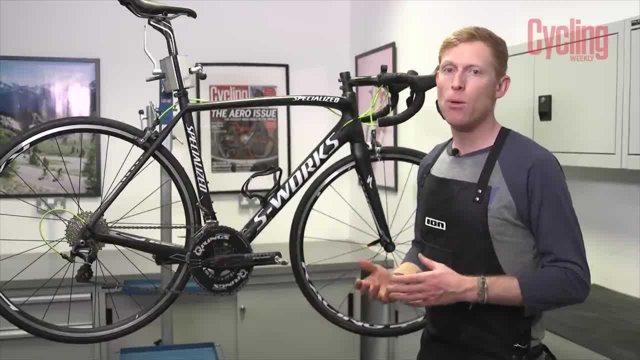 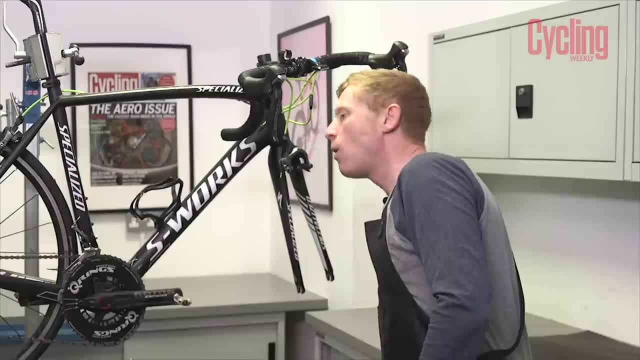 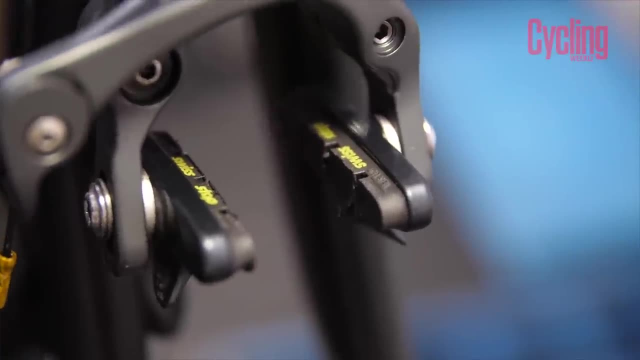 With both types of bikes, it's better to do it with the wheel out. So, if we take your wheel out, what we're looking for is we're looking for any wear on the pads themselves. Now, most pads for rim brake will have little channels in them, and these can act as wear guides. So, if you can see, 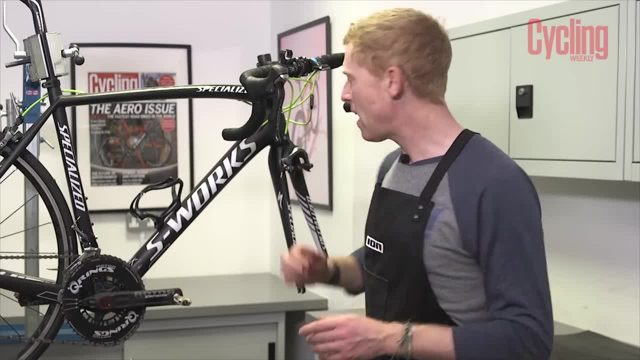 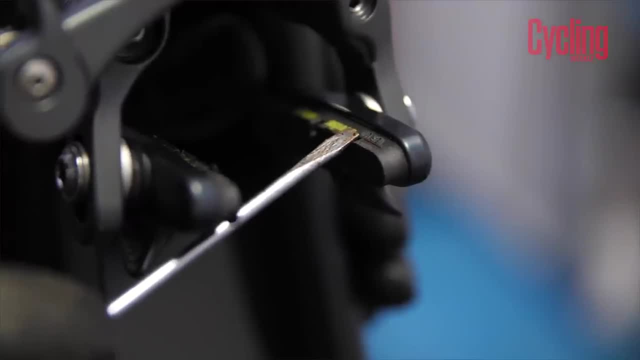 the channels, then often that is fine. Now, these pads, these are Swiss Stop pads and they've got a wear line on them, So I can inspect that visually to make sure that it's actually still got plenty of life, which they do, which is good. And then the other thing to look at is to look to 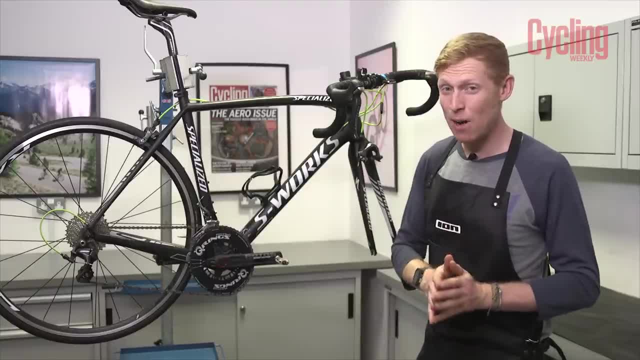 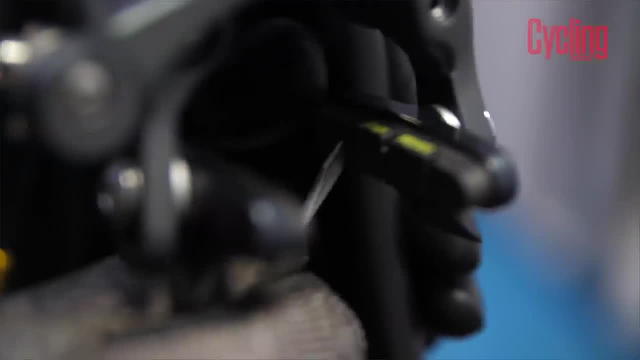 see if there's any debris impacted in the pad material itself. Now what you will find is that the rims will shed metal, So you can end up with little spots of aluminium in the pad material itself. So you can use a small screwdriver to get rid of any of that, and some sandpaper if 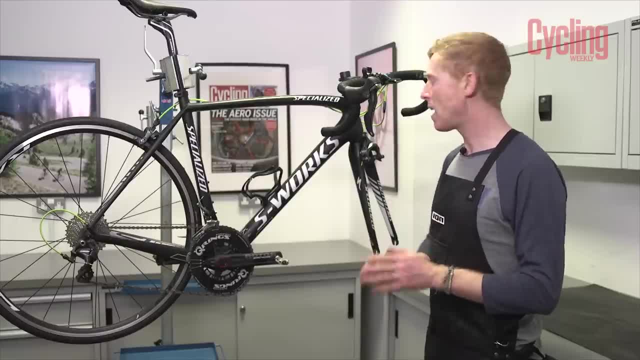 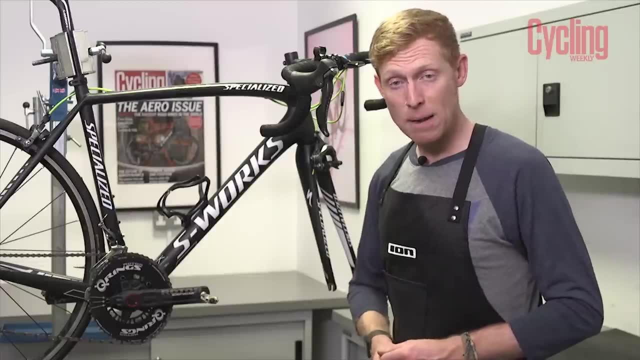 you want to, to get a really, really good job, to get those nice and smooth again With your disc brake pads, then the same applies. You want to be checking the pad material to see that there's enough pad material there and to make sure that the pistons themselves are working properly. So 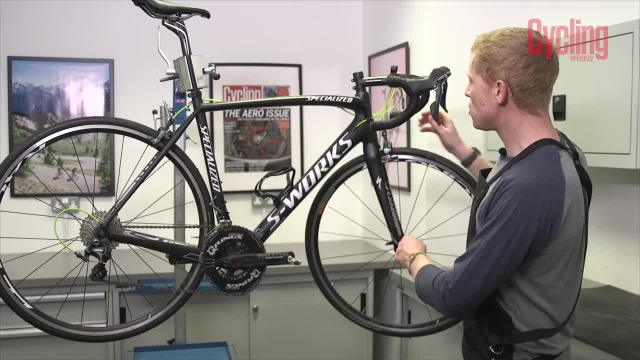 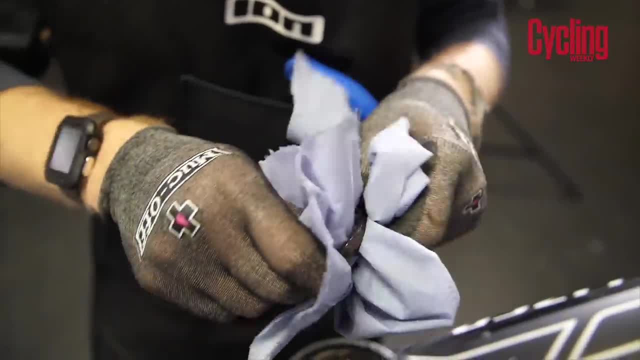 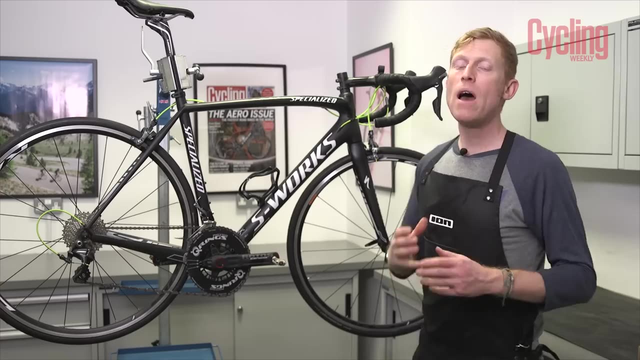 moving up from there. obviously you have the headset, So the two bearings that allow your bike to steer. Now these can have lots of problems, especially over a really hard winter like we've had, And what you might find is especially the bottom bearing here that can develop a lot of play. 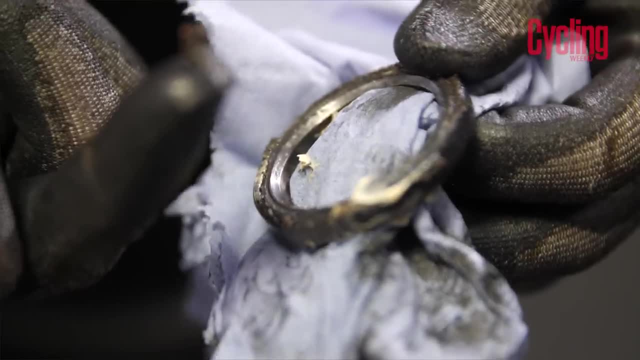 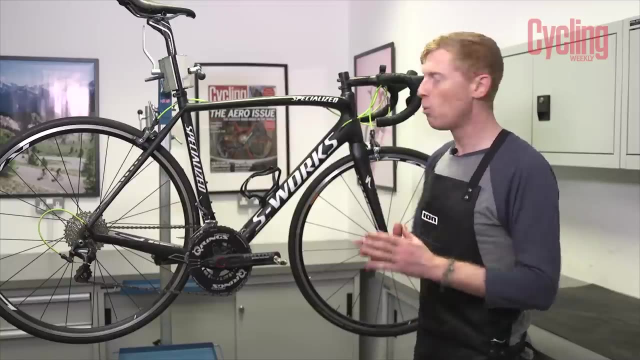 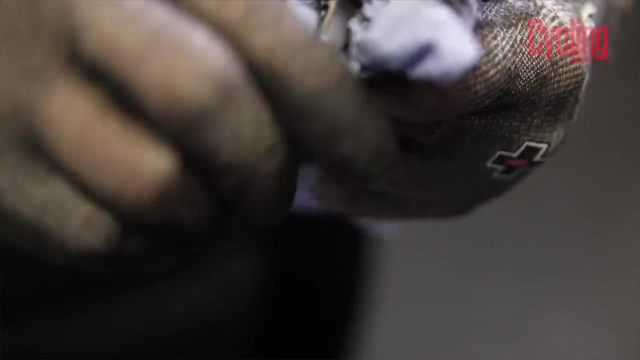 or it can feel very, very notchy and horrible because at the end of the day, it gets a lot of dirt, a lot of grime in this. You want to be able to inspect these bearings, So you will want to take the headset apart, check the bearings themselves and, obviously, to clean and re-grease. 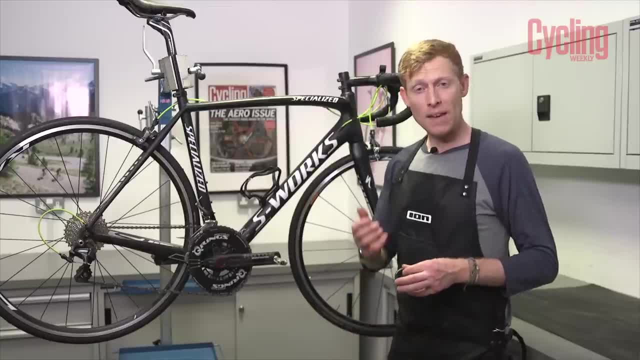 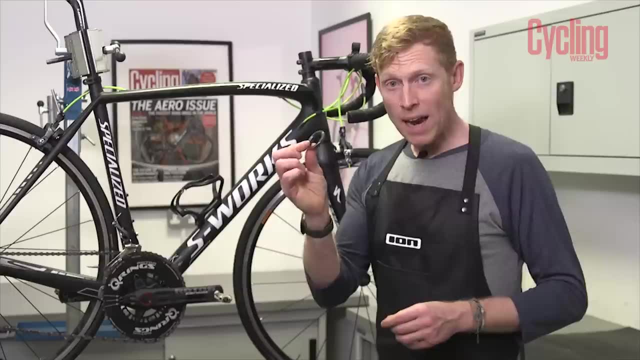 those. Now, if you find that your bearings are damaged or there's too much grunge and grit in there and you want to replace them, then you need to make sure you're getting the right bearings. So when you take your headset bearings out, 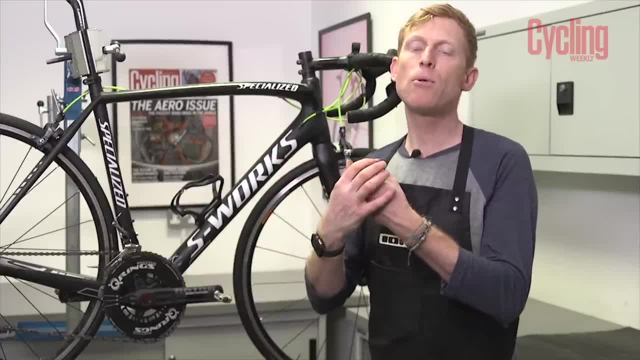 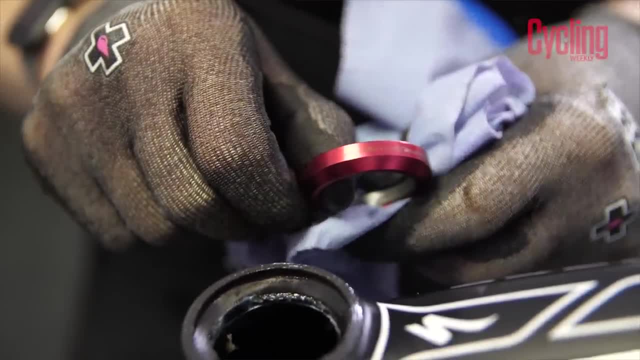 you'll find that on the side of the bearing there should be printed not only the name, but some numbers on there. These will correspond to the exact type of bearing you require And for most bikes with tapered headsets. don't forget that both top and bottom will be very, very. 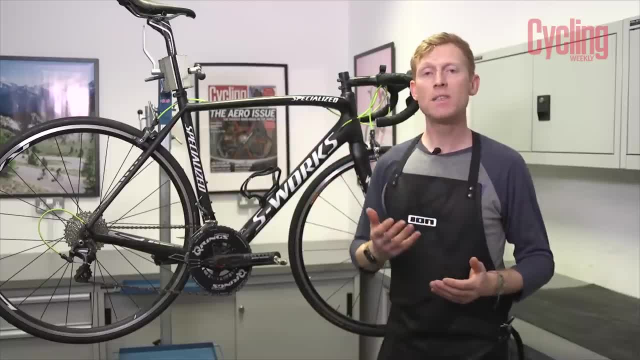 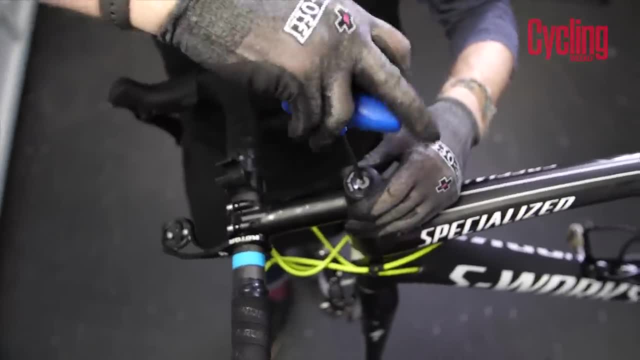 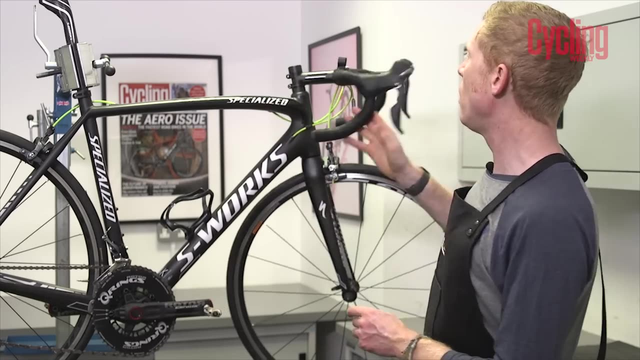 different Moving upwards. we've got, obviously, the stem and the handlebars, So it's critical that your stem bolts are tight and that they are evenly tightened as well. So make sure you check not only the two stem bolts at the back, but also the stem bolts that hold your 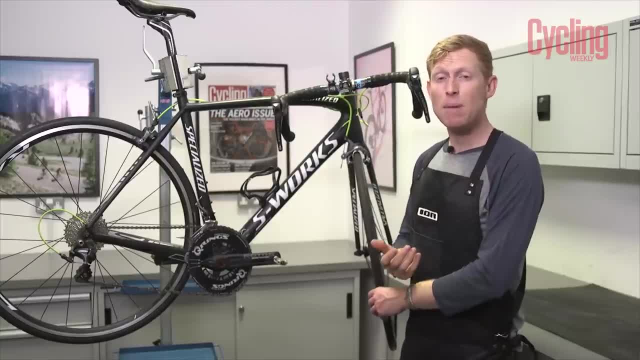 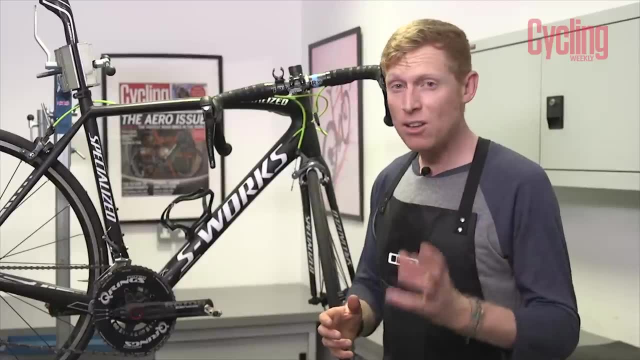 handlebars in place, If need be. if you're finding that there's a bit of noise when you're riding your bike, you might want to take those out individually and clean and re-grease them. That is a good top tip for making sure that it gets rid of any clicking or creaking noises from. 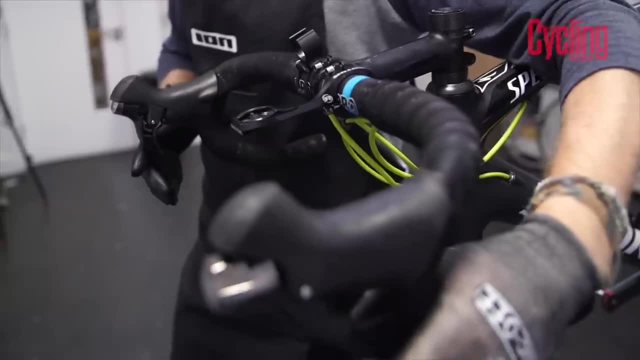 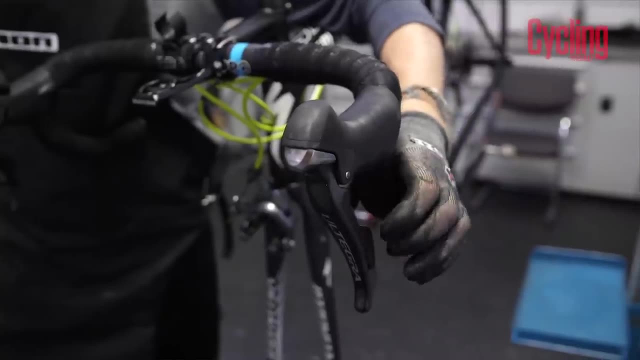 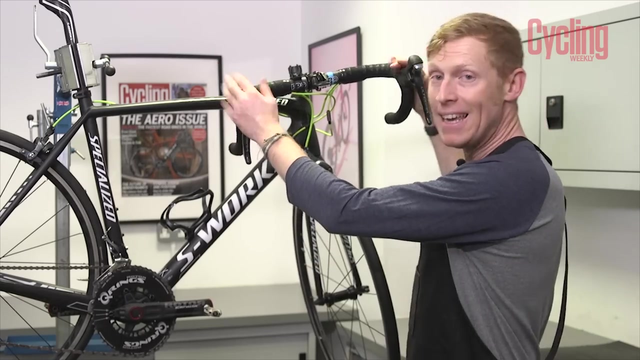 here. once you've eliminated other parts, Then you need to go and look at your shifters. So you want to make sure that your shifters are in place, that they're in place freely and that they shift as well as pulling the brakes, And, obviously, that they are in the right place at the right angle. 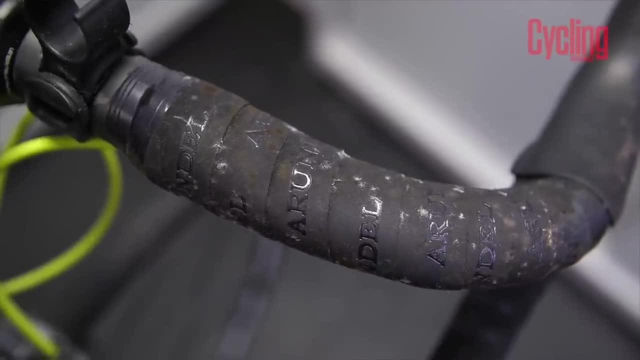 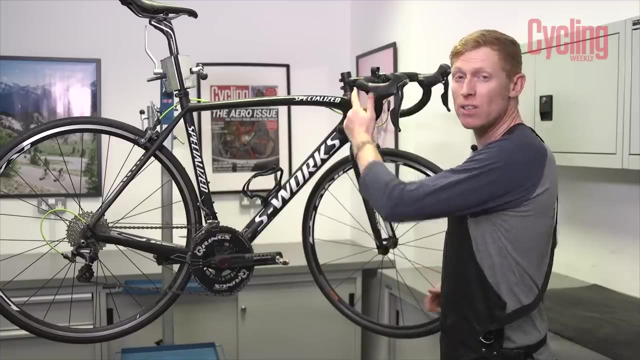 and that they're both even. And the final thing with the cockpit area is obviously your handlebar tape. Now mine, sadly, has seen the last of its useful life. It was covered in mould. Not only that, but it's also worn through here as well, So there's less grip. So I do need to change this bar. 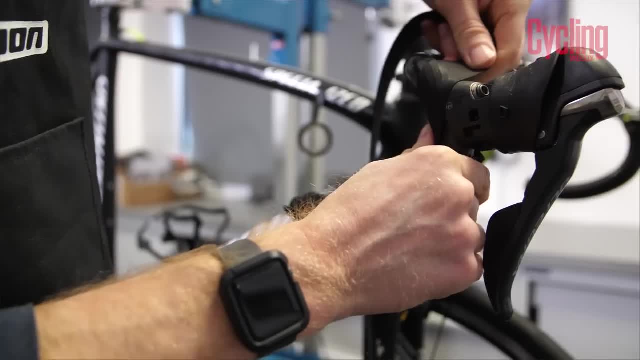 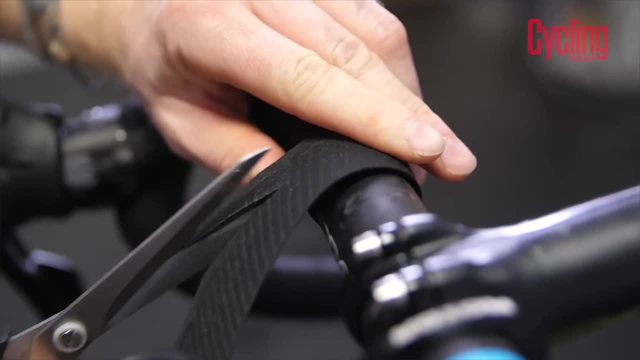 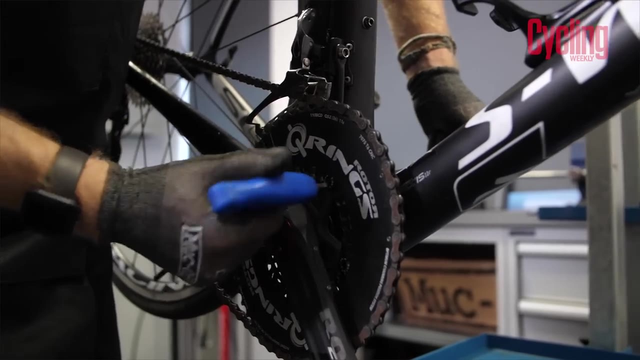 a little bit to make sure that it's in the right place. Now we're going to bring it down to the bottom bracket area, So we're talking about bottom bracket bearings and chain set and front derailleur as well. So first thing you need to do is to make 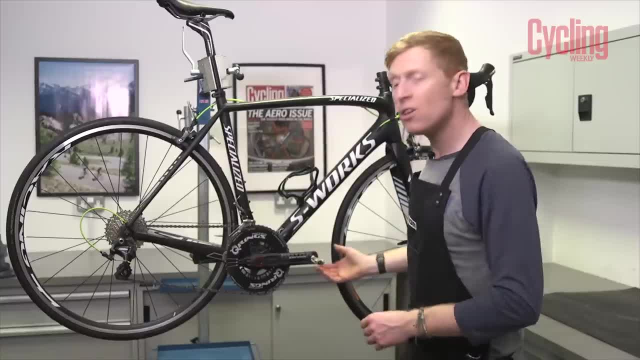 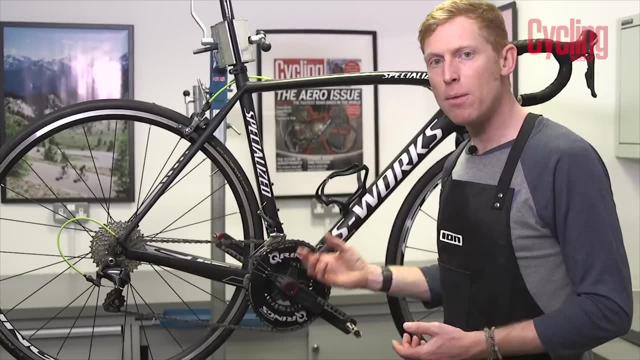 sure that your bottom bracket is working properly, So give it a spin Now. you can do this with the chain on to start off with, but it's also really important to make sure that the chain is in place as well, So it's really really good to do it without the chain. This will give you an idea as to how freely 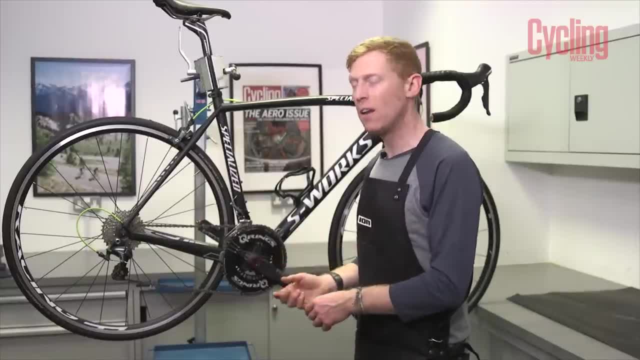 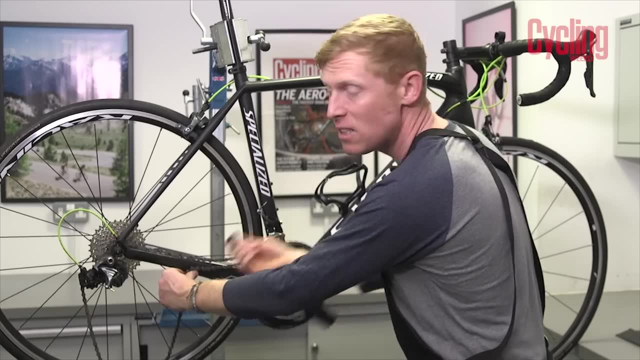 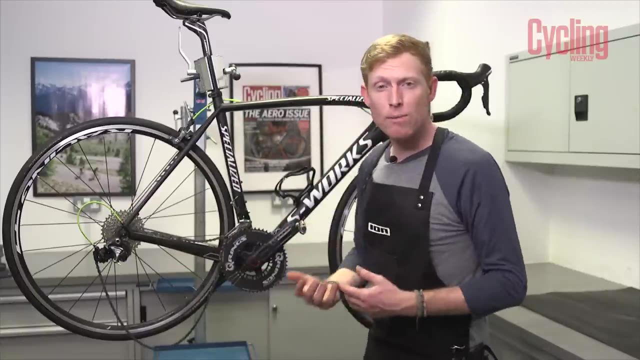 it actually is spinning. So very simply, you can derail the chain over the front like so, So you can spin this nice and freely and work out if there is any play in that bearing or also if it feels very, very tight and stiff. If that is the case, then you might need to be. 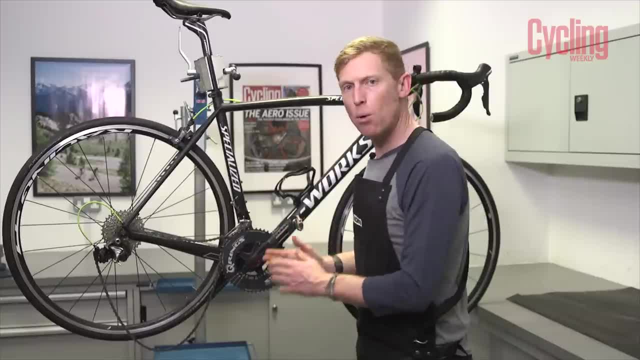 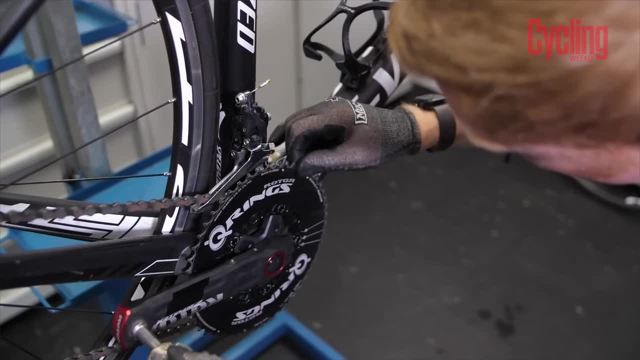 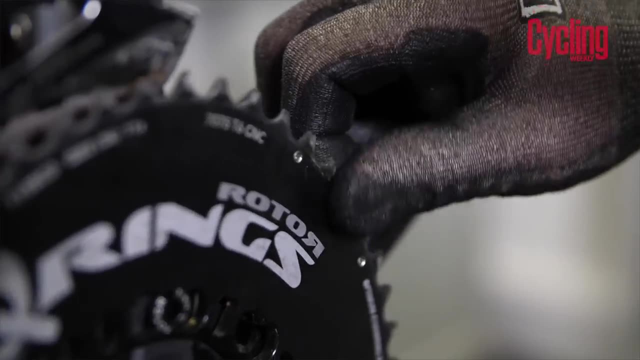 replacing this bearing as well, And again, that's a real important part of the bike, So you need to make sure that's done properly. Then we're going to visually inspect the chain rings to make sure that the chain rings themselves have enough life left in them to keep going on the bike. So we're looking at tooth profile here. 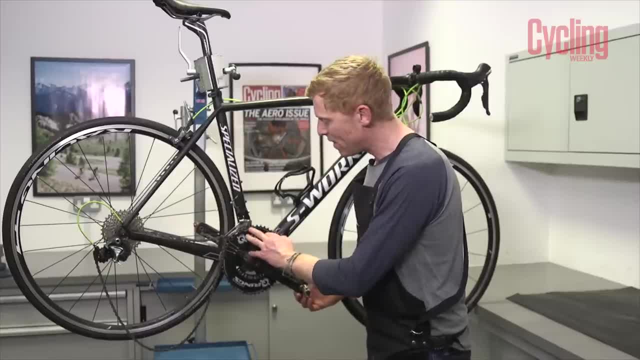 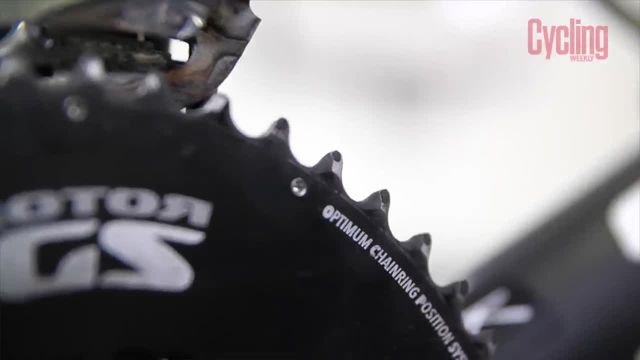 So we want to make sure that they're not too sharp and too pointed and that the gaps between them is even So, making sure that they look natural and even and how a chain ring should look. Check the chain ring bolts as well. Make sure everything is nice and tight. There's nothing worse. 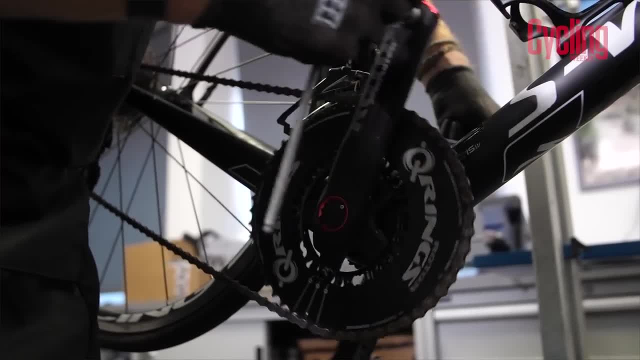 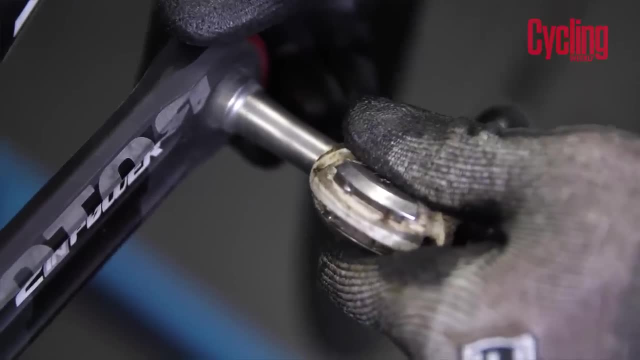 than losing the chain ring bolt while you're out and then you can't continue your ride While you're down here as well. check your pedals, So we're looking for any play in the pedals themselves and to make sure that the mechanism is working properly And these are actually doing. 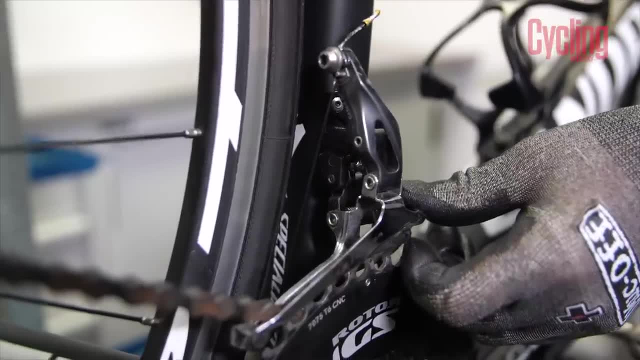 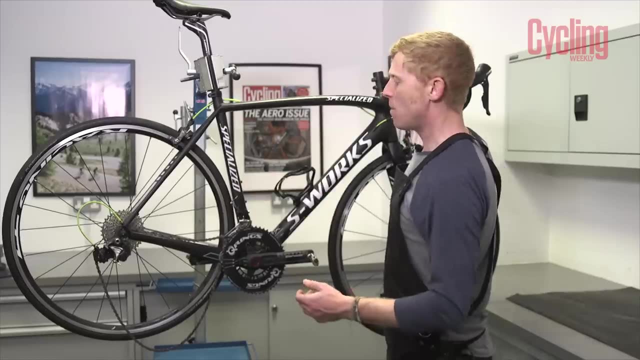 really really well at the moment, which is good. Then, finally, while we're still down in this spot, check your derailleur. We are looking for any excess play where they shouldn't be and also making sure that it's working properly, so that the cable is working. There's no. 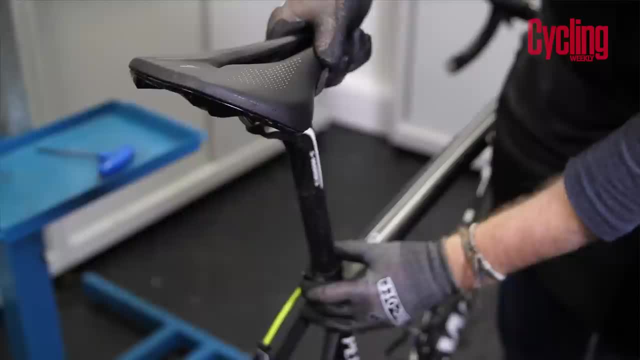 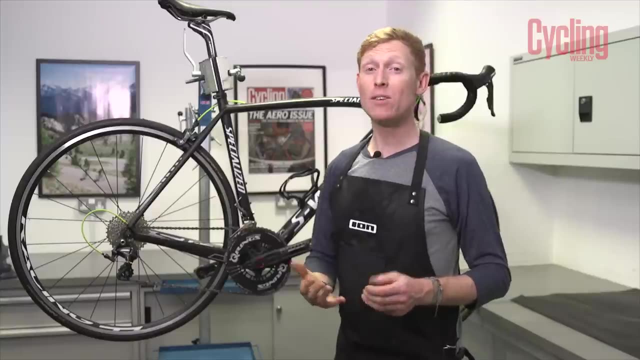 damage to the cable and that everything is nice and tight. Moving on up the fourth point, we're talking about your seat post and your saddle. What we're making sure of here is, first of all, you can take it out so it's not seized, And then, secondly, you need to re-grease that. 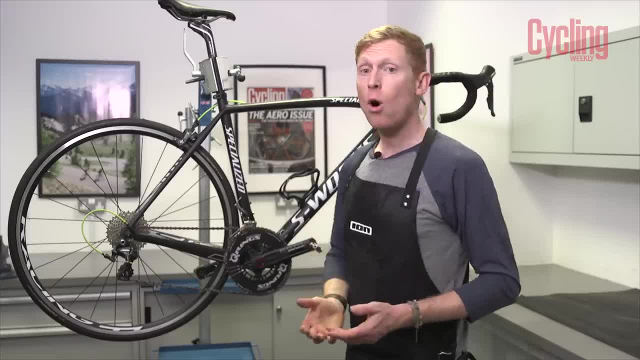 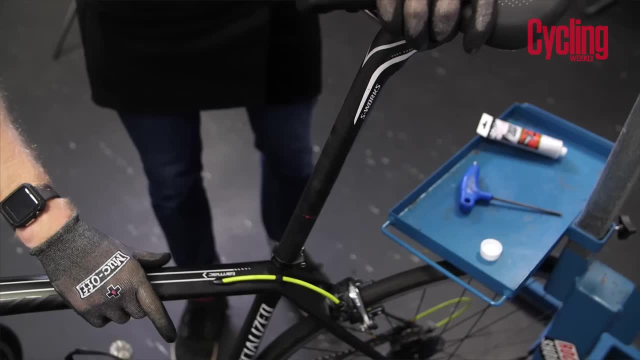 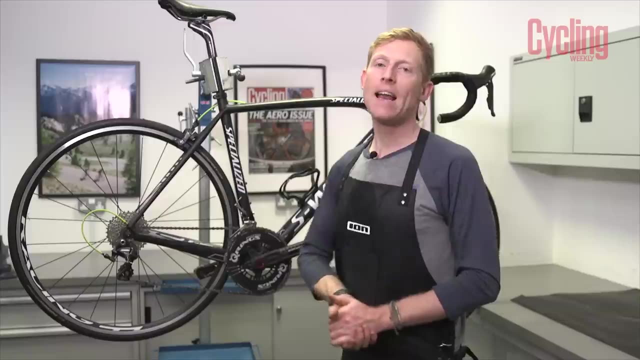 seat post. So making sure you're either using normal grease or something like fiber grip, which is an anti-slip that is required when you use a carbon seat post. This means that you don't have to worry too much and everything will stay nicely in place. Now, one of the things that can 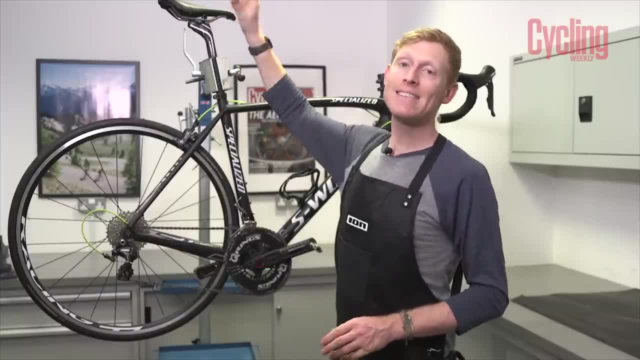 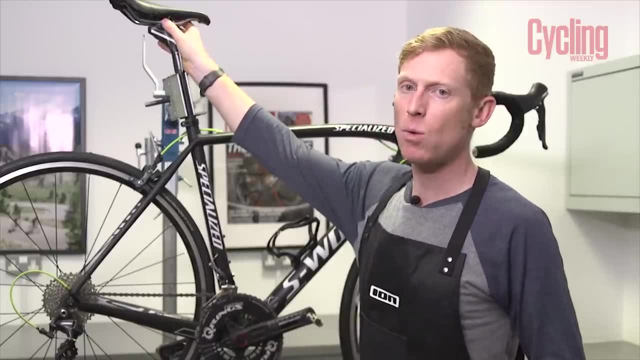 happen over time is your saddle rails or your saddle itself can start creaking. So we want to make sure that this is working properly and that your saddle is clamped properly as well. So you might want to take off your saddle, re-grease the rails where they actually sit. 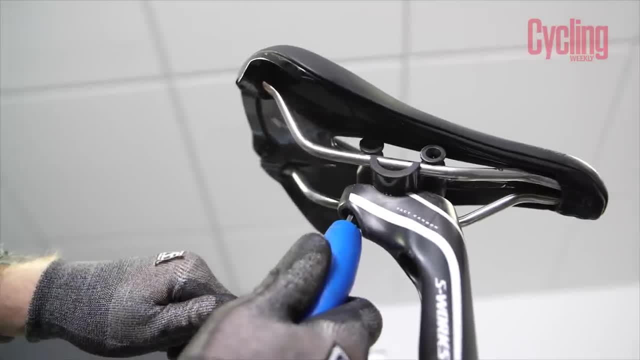 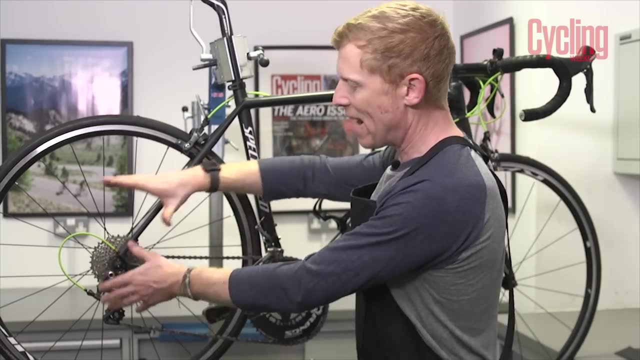 in the clamp itself, and then make sure you've done it up properly. Finally, we're going to come down to probably the busiest part of the bike, Down at the rear axle area. Again, we've got a wheel to think about, So go through the same. 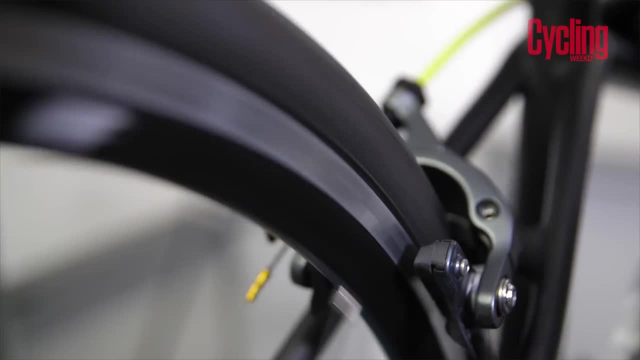 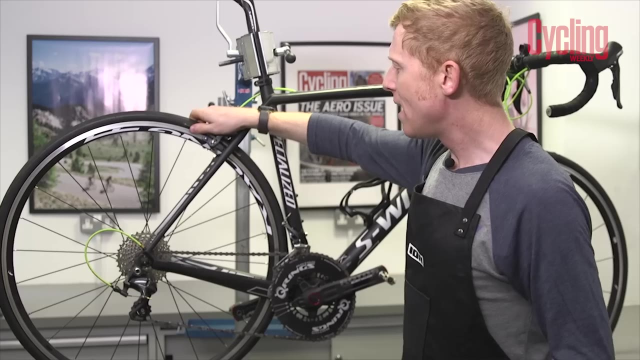 inspections you did with the front wheel. Spin the wheel, make sure it's running nice and true. If not, then get that trued And then again check those hub bearings as well. Now, here we've not only got two hub bearings, but there are also two bearings in the free hub as well. 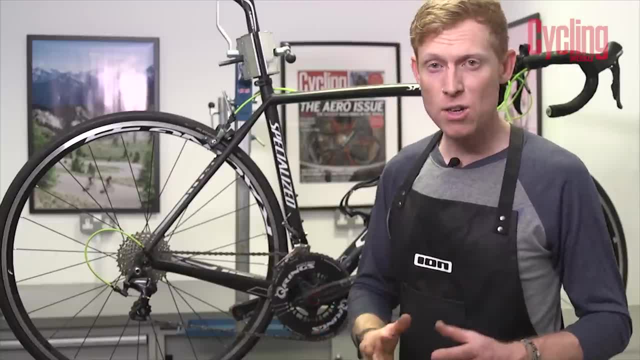 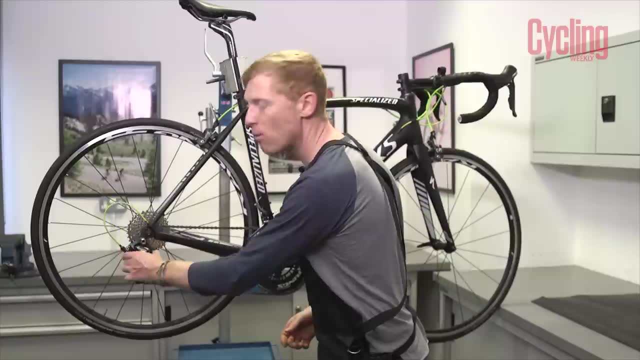 So there's four to think about. You might find that only one is gone, but that can cause a lot of problems If we go down to the derailleur. first of all, we want to make sure it's functioning properly, So you can do this by moving it around yourself and, of course, 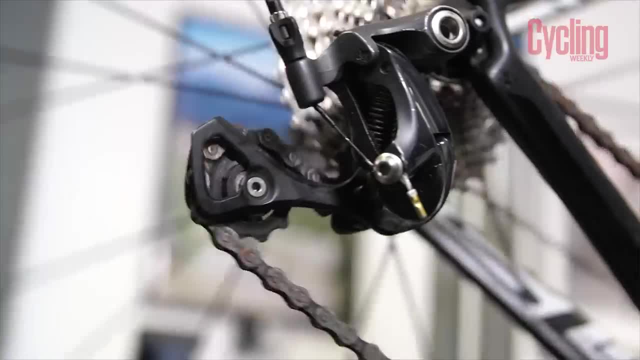 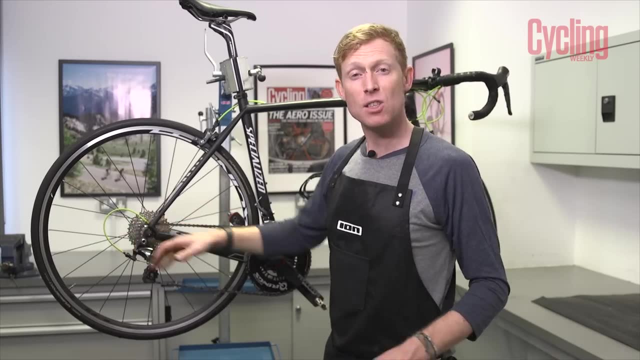 by shifting gear. So if we shift gear we can work out if it is working properly or if it needs any adjustment whatsoever. Now this one seems to be working nice and smooth Again. with that lever action you can feel to see if there's any roughness in the cable itself. 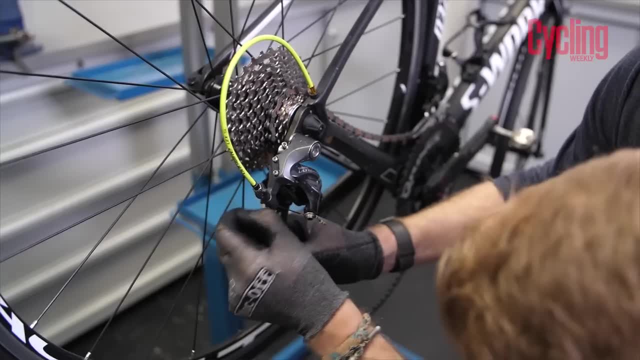 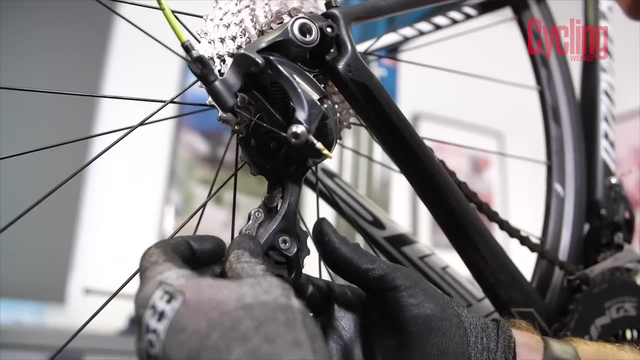 And if there is, then you might want to be replacing the cable as well. Check your jockey wheels or your pulley wheels for any excess. So we're looking at the teeth on the jockey wheels here and making sure that they're not too pointed, which can happen over. 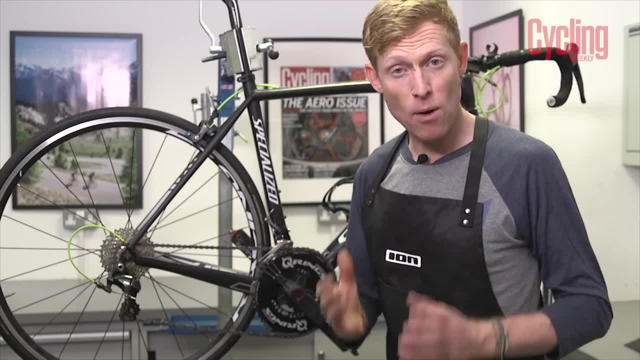 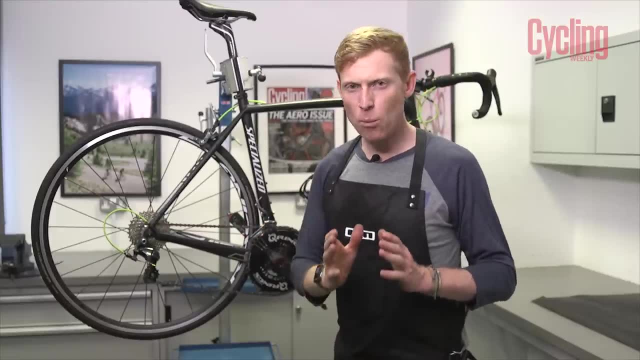 time. And then look at your cassette. We're looking for any excess wear on any of the teeth, same as we've done with the chain rings themselves. And finally, probably the one thing that we'll need replacing out of everybody's bikes is the chain. Now mine looks horrible. 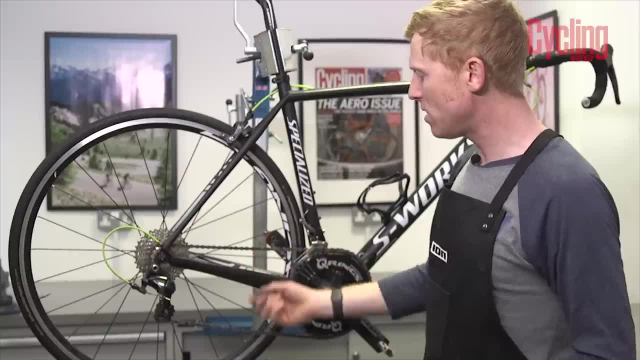 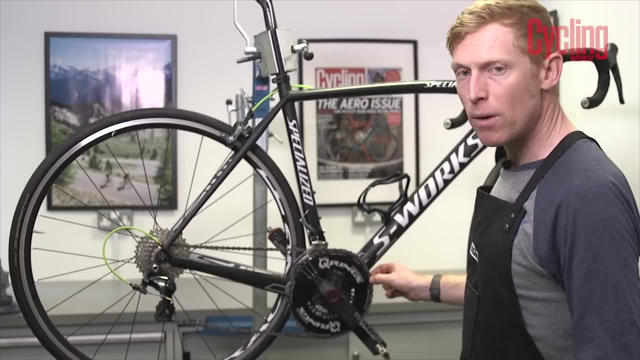 It is a bit rusty, It's a bit grunchy And the worst thing is, if you move it, you can move it a lot of side to side here And if you put it over here you can actually see it comes away from the chainring. So this is some of the 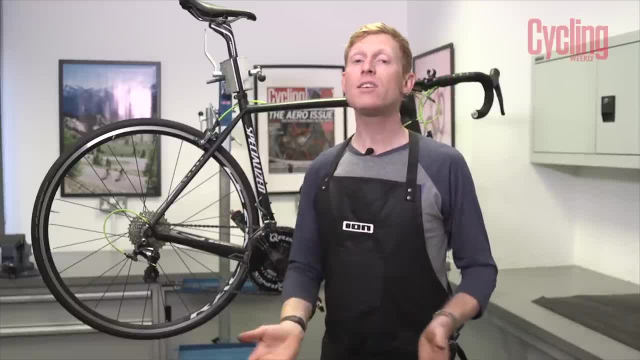 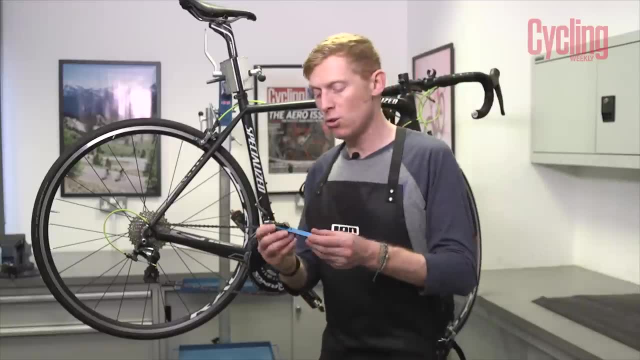 indicators that it is worn. If you want to do it properly, though, you need a chain checker- something that's very, very inexpensive, but something that is really, really handy to have. I've got a Park Tools one here, which is actually really simple to use- Two little prongs- So we 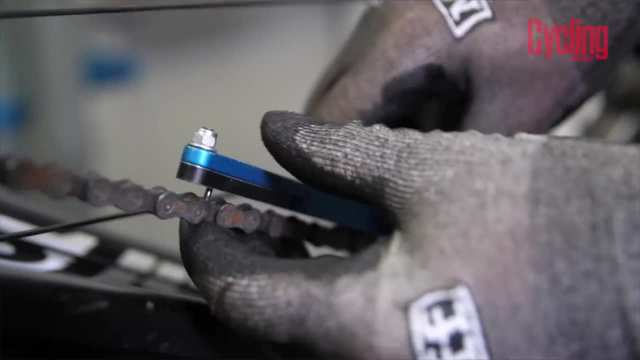 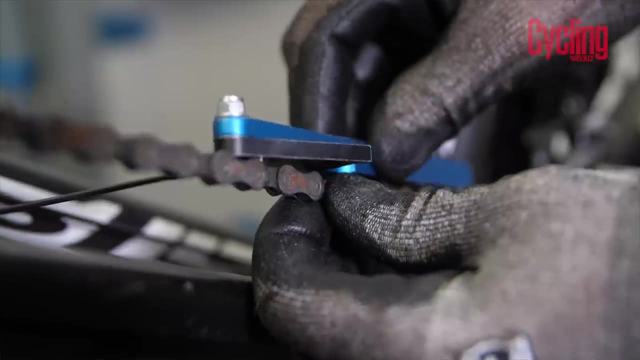 just put it on top of the chain, like so. So we put it through one of the chainring links and then through the other one, like that, And then you push this little black part here and this will tell you how worn the chain is Now. actually.